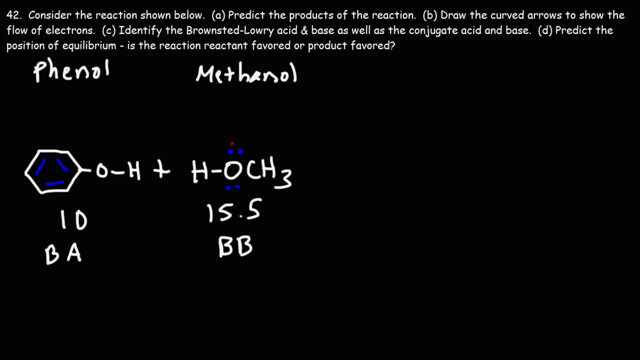 So the base is going to be like the nucleophile: The arrows are going to point from the lone pair to the hydrogen. Now, when this bond breaks, where does it go? Where would those electrons go? Are they going to go towards the oxygen or the hydrogen? 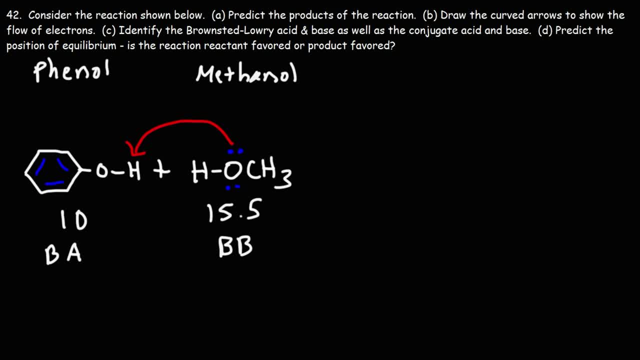 They're going to go towards the element that is more electronegative, In this case that is oxygen. Oxygen is more electronegative than hydrogen, So when that bond breaks, these electrons go back to the O, So we're going to get the conjugate base of phenol, which is phenoxide. 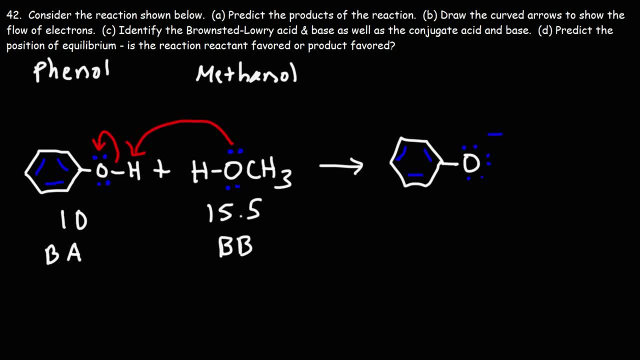 And it's going to have a negative charge And we're going to add the hydrogen to methanol, giving us the conjugate acid of methanol. So anytime you take away a hydrogen, you're going to create the conjugate base. 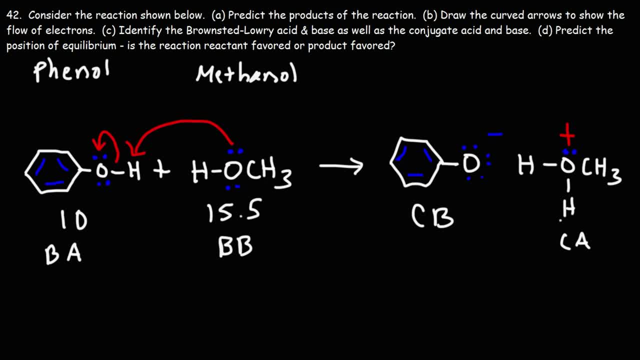 When you add a hydrogen, you're going to get the conjugate acid And basically we've completed part C. Identify the brancelari acid and base, as well as the conjugate acid and the conjugate base. The conjugate acid is the acid on the right. 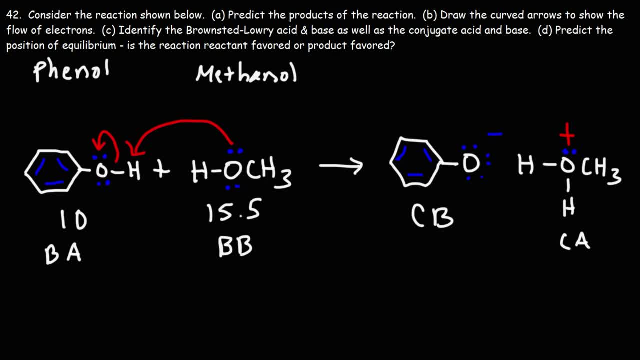 The conjugate base is going to be the base on the right side, The brancelari acid and base that's going to be on the left side of the reaction. So far we've finished part A, B and C. Part D predict the position of equilibrium. 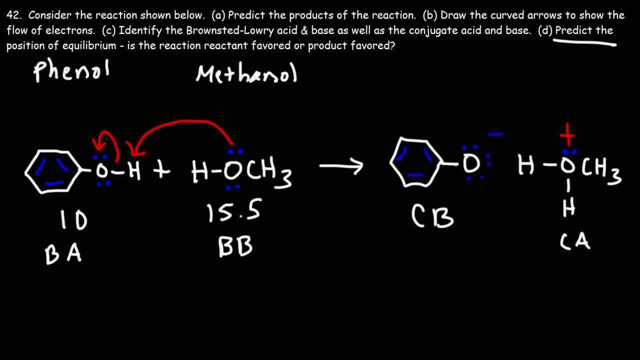 Is the reaction reactant-favored or product-favored? What would you say? In order to figure this out, we need to look at the pKa values of the brancelari acid and the conjugate acid. So what is the pKa of a protonated methanol? 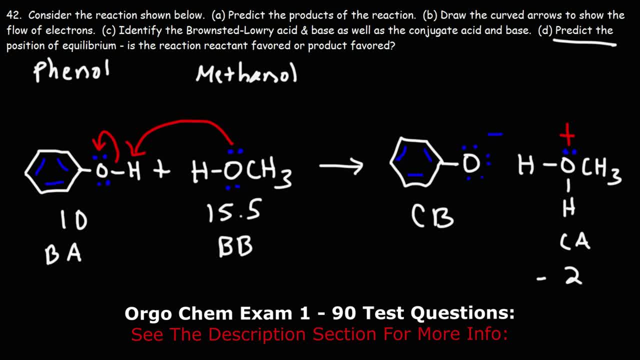 If you recall, it's around negative 2.. Now, comparing these two acids, which one is stronger and which one is weaker? The stronger acid has the lower pKa. The weaker acid has the higher pKa. The��アカレ vek qué 64007 atyp. 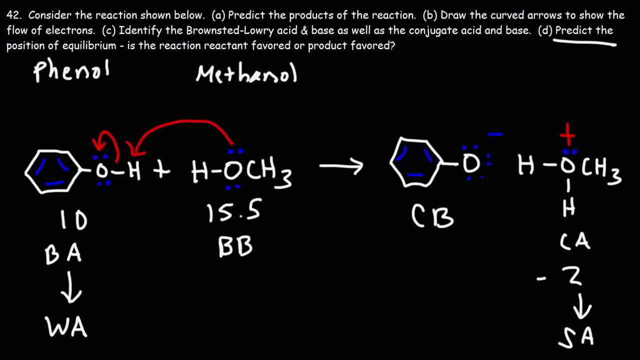 The position of equilibrium, reactions tend to proceed in a way such that they create more stable products. Think of a ball rolling down a hill. the ball wants to go down to a lower energy state, a state that's more stable. The ball won't naturally go up the hill to something that's less stable or to a less stable place. 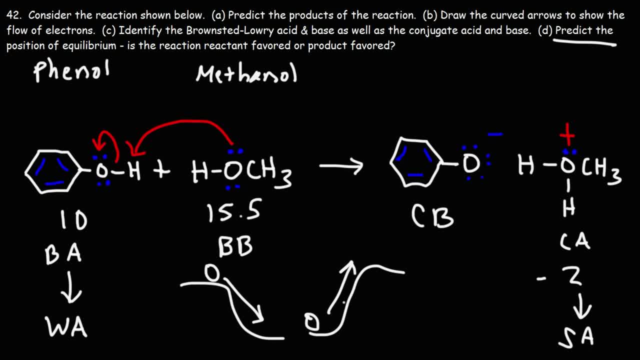 position, unless you apply energy, of course. so things naturally tends to go down the energy profile, so objects tend to go from a high energy state to a low energy state. that's the general trend. so this reaction is going to proceed in a direction that produces the more stable acid. the more stable acid is less. 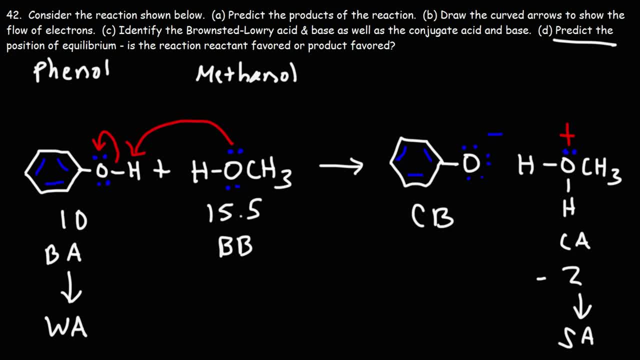 reactive, it has a less potential energy. in other words, the more stable acid, the less reactive acid is the weaker acid. so it's going to go to the side with the weaker acid and the weaker acid is on the left side. so this reaction is reactant favored. here we have separation. 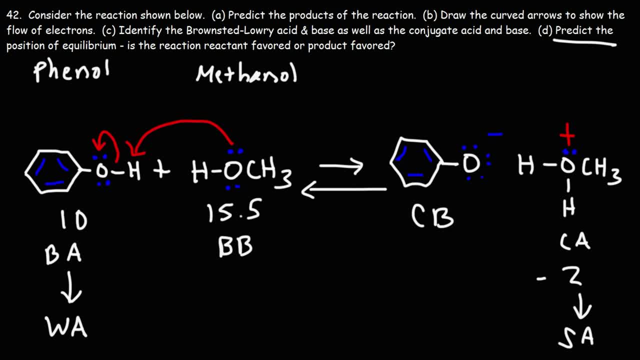 of charges. so that's a good example of a reaction that produces less potential acid compared to a reaction that produces less defense�. that indicated that it's probably not going to be a product favored, even though that's not always the case. there are exceptions, but we're creating a very 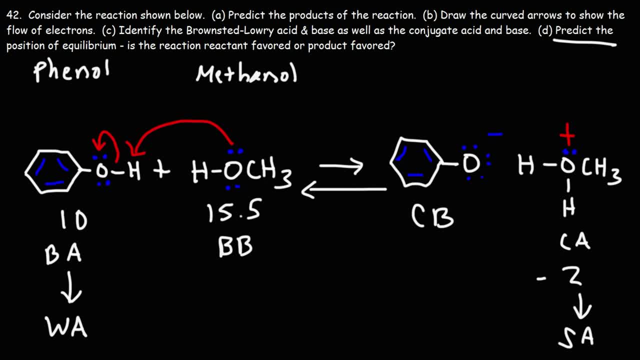 reactive strong acid and either has relatively significant base. so if we were to put phenol and methanol in solution, less than one percent will be in this form. So that's the key. Okay, so that's a good definition here. how have we defined this important base? 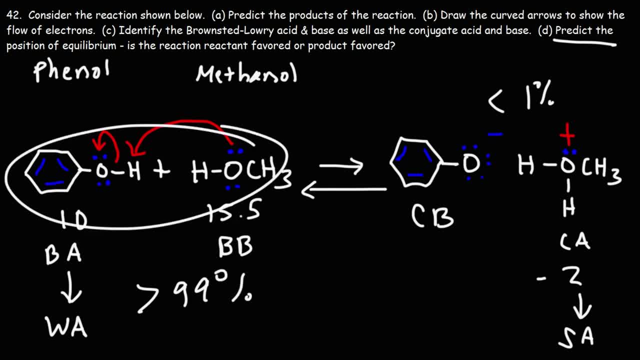 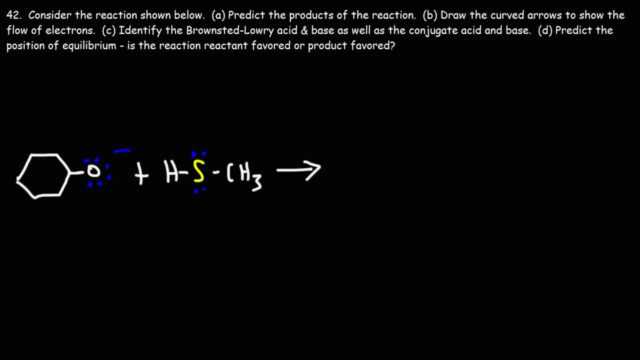 More than 99% of the molecules will be in this form, but a small amount will react to create these products. but it's going to be very, very small. Now let's move on to the second example. So we should probably start with the first half of part C. Let's identify the brancelaria. 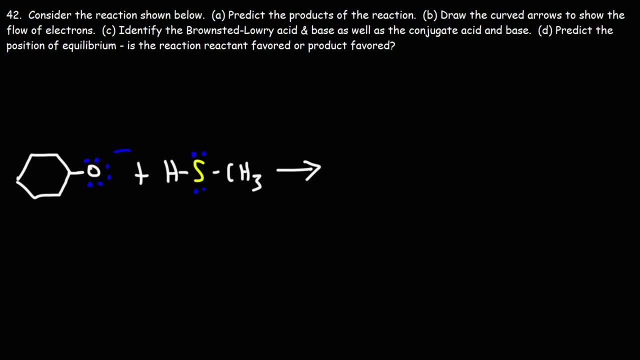 acid and a brancelaria base. So here we have an alkoxide ion- It's the conjugate base of an alcohol- and here we have a thiol. We know the pKa of a thiol: it's 10.. Now, because this has a negative charge, it's most likely to act as the brancelaria base. 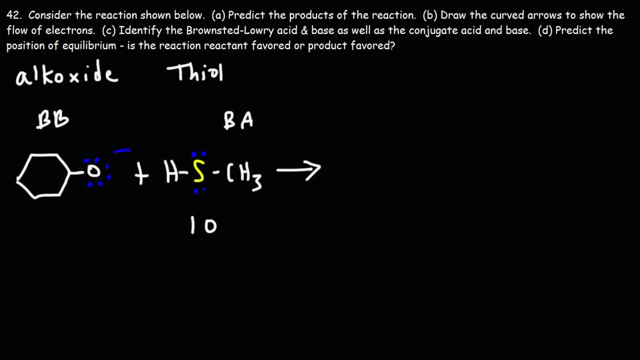 The thiol is most likely to act as a brancelaria acid. I mean, like, if you think about how else we can do this, there really isn't another way. I mean, If we want sulfur to act as a base and to take off this hydrogen, that's likely not. 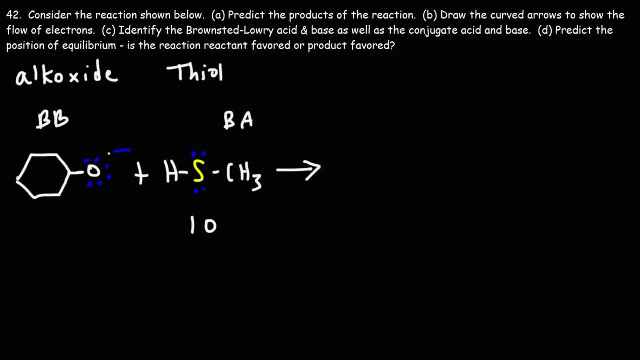 going to happen, So it's safe to assume that this is going to be the brancelaria base. It wants to get a hydrogen and this has a hydrogen to give away, So that's going to be a brancelaria acid, the proton donor. 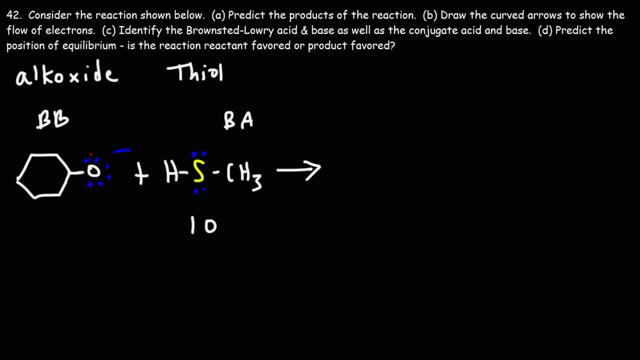 So let's draw the curve arrows to show the flow of electrons. So we're going to start from base to acid, and when this bond breaks, hydrogen has an electronegativity value of 2.1, sulfur is 2.5.. 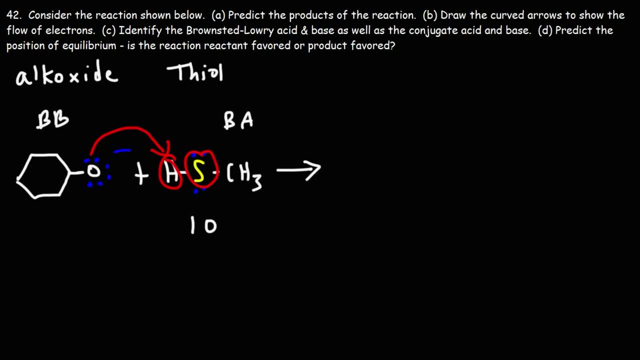 So sulfur is more electronegative than hydrogen. So when the SH bond breaks, those electrons will go to the sulfur atom. We're going to get the conjugate acid cyclohexanol and the conjugate base of the thiol, which 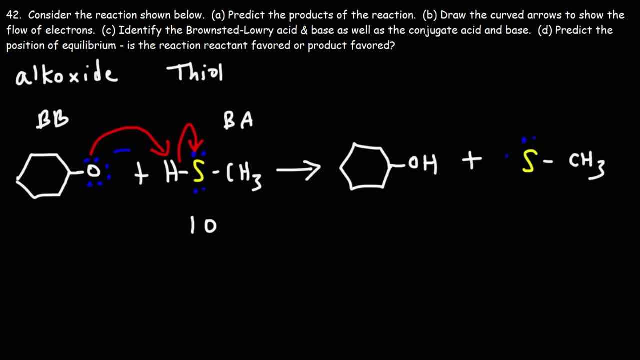 will look like this. So this is the conjugate acid. this is the conjugate base. Now the pKa for cyclohexanol is 18.. So far we've completed part A. We've predicted the products of the reaction. 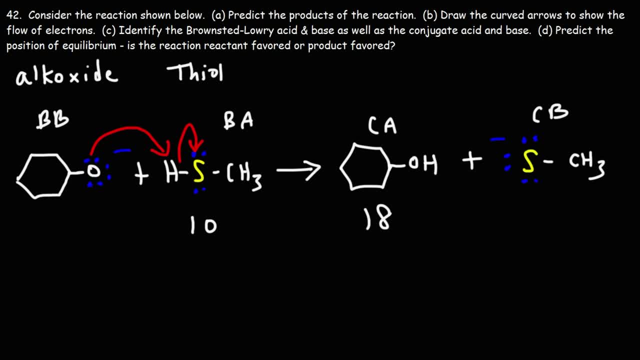 We got cyclohexanol and the conjugate base of the thiol. We drew the curve arrows to show electron flow And we've identified the brancelaria acid in base as well as the conjugate acid in base. So now we need to predict the position of equilibrium.